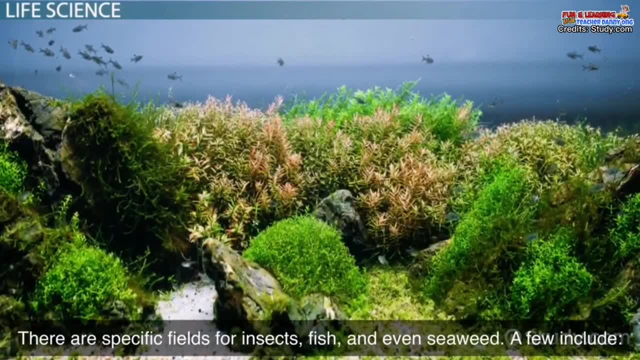 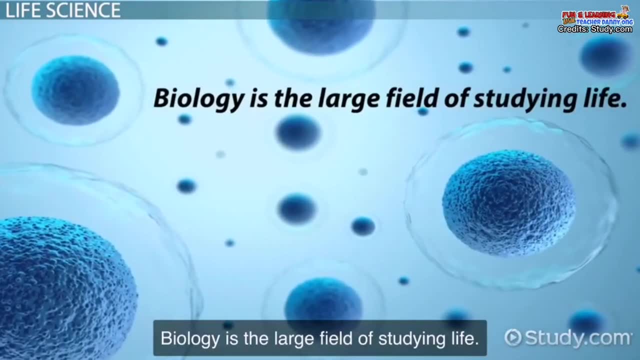 what living thing you decide to study. There are specific fields for insects, fish and even seaweed. A few include…. Biology is the large field of study of life. Here you can study all sorts of living things and how they interact with one another. 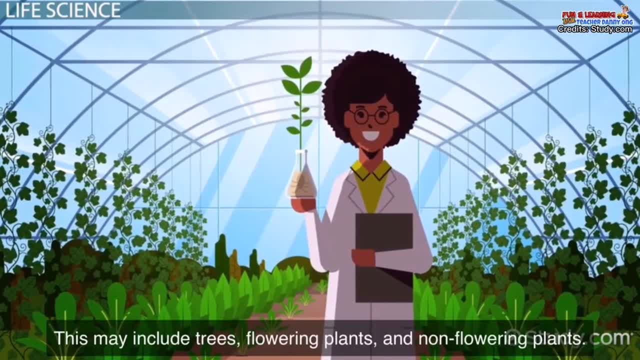 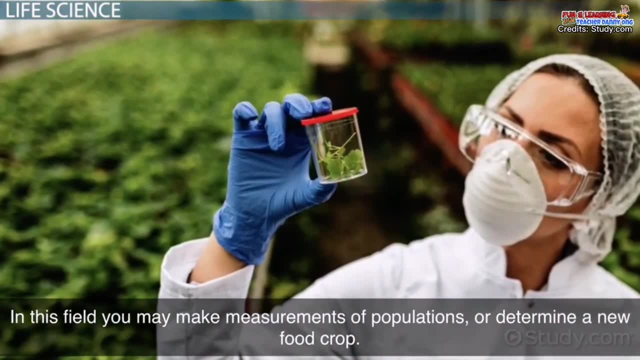 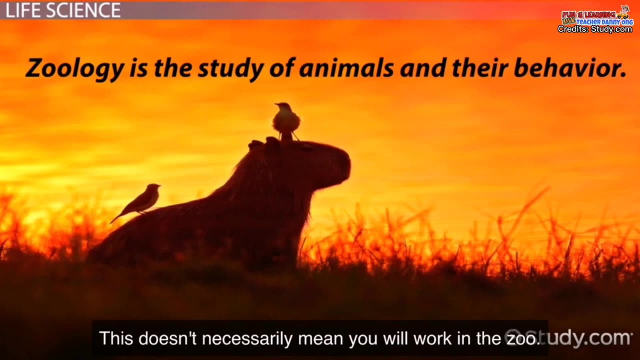 Botany is the study of plants. This may include trees, flowering plants and non-flowering plants. In this field, you may make measurements of populations or determine a new food crop. Zoology is the study of animals and their behavior. This doesn't necessarily mean. 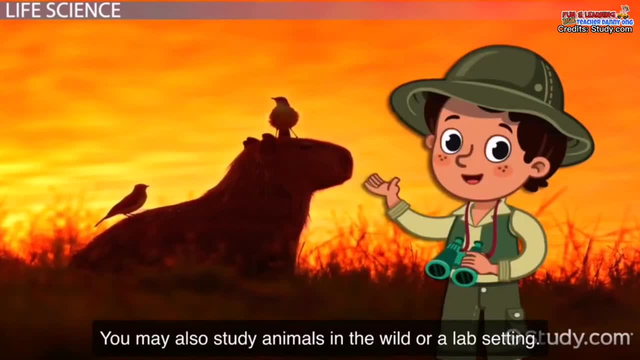 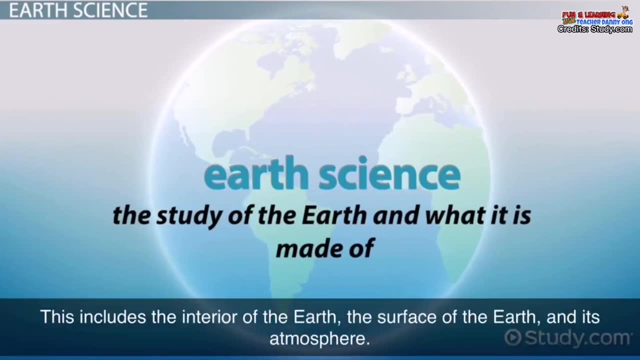 you will work in the zoo. You may also study animals in the wild or a lab setting. Earth science is the study of the Earth and what it's made of. This includes the interior of the Earth, the surface of the Earth and its atmosphere. There are many fields of study. 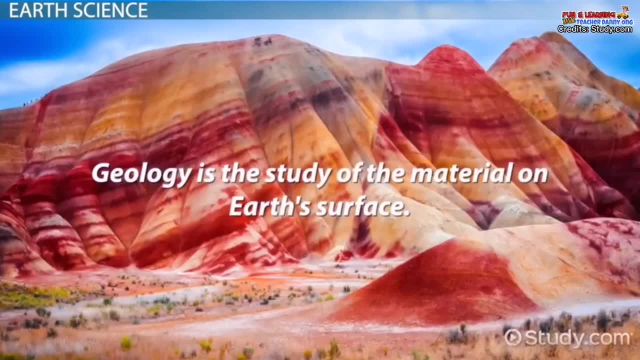 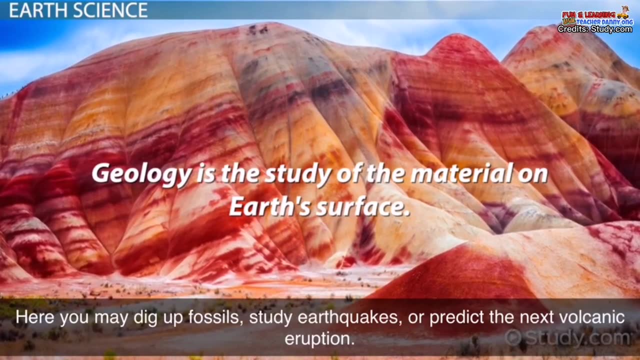 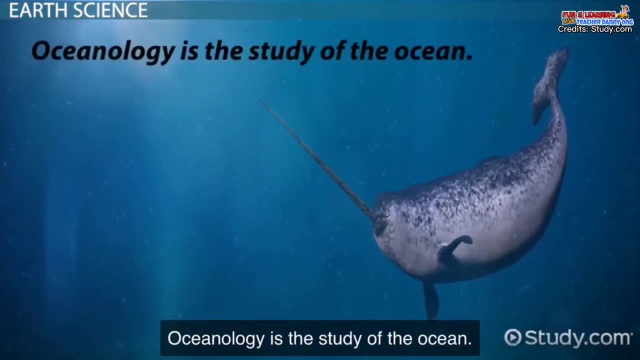 in this branch as well, but here are a few. Geology is the study of the material on Earth's surface and events that take place there. Here you may dig up fossils, study earthquakes or predict the next volcanic eruption. Oceanology is the study of the ocean. Remember this would not be the living thing. you would. 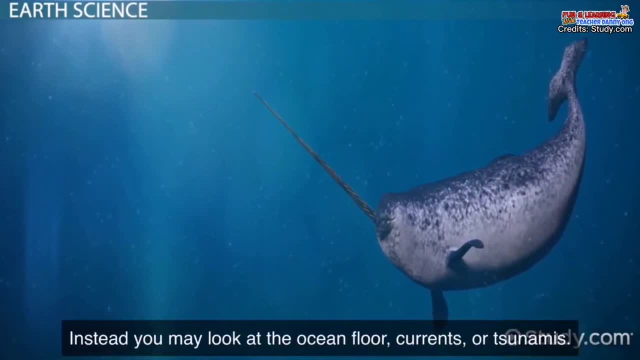 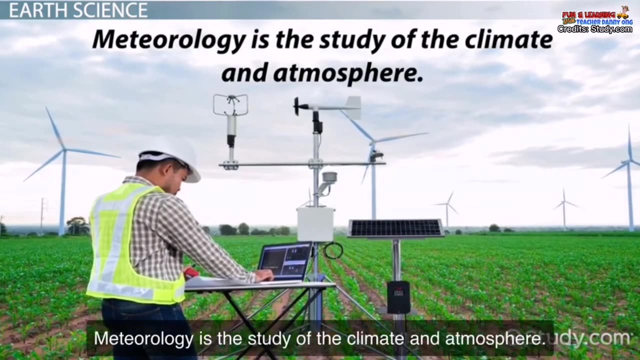 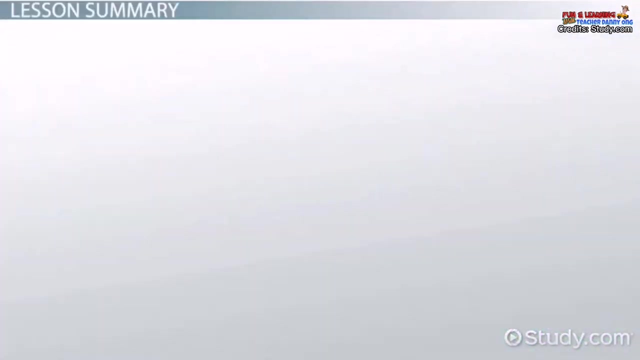 see in the ocean. Instead, you may look at the ocean floor, currents or tsunamis. Meteorology is the study of the climate and atmosphere. This includes predicting the weather, measuring climate change and predicting the impacts of each. 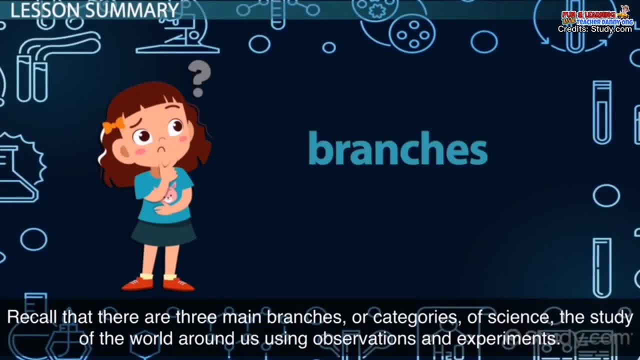 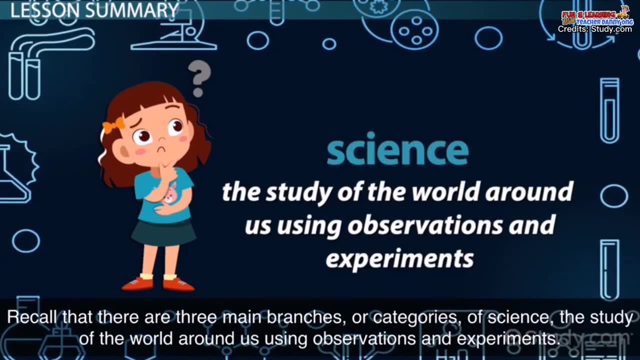 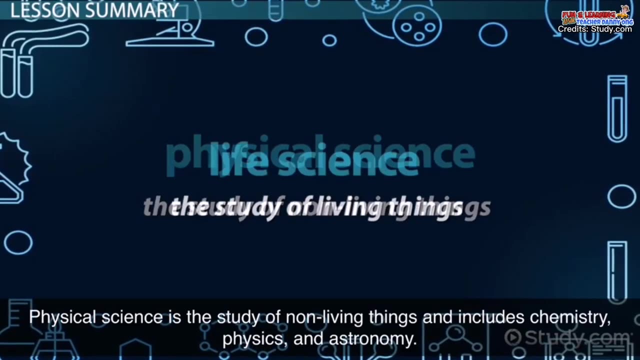 Have you decided which one is your favorite? Recall that there are three main branches or categories of science: the study of the world around us using observations and experiments. Physical science is the study of non-living things and includes chemistry, physics and astronomy. Life science is the study of living things and includes biology, botany and zoology. 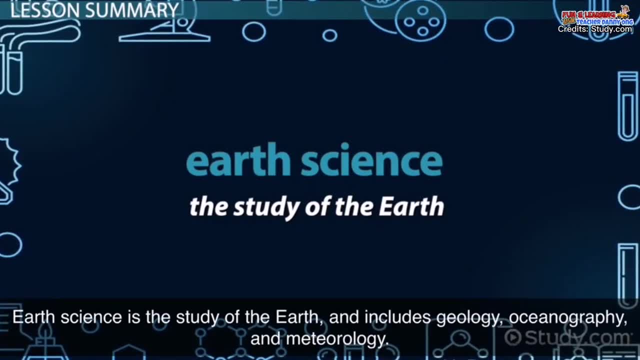 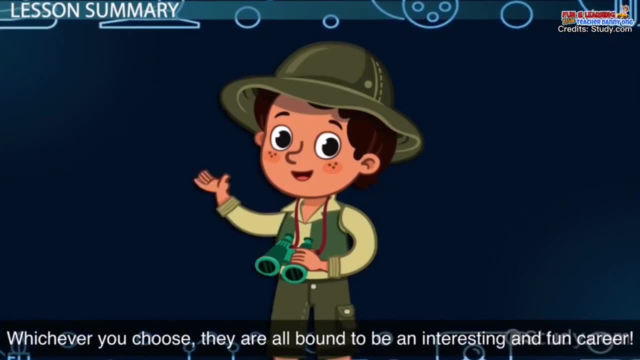 Earth science is the study of the Earth and includes geology, oceanography and meteorology. Whichever you choose, they are all bound to be an interesting and fun career.